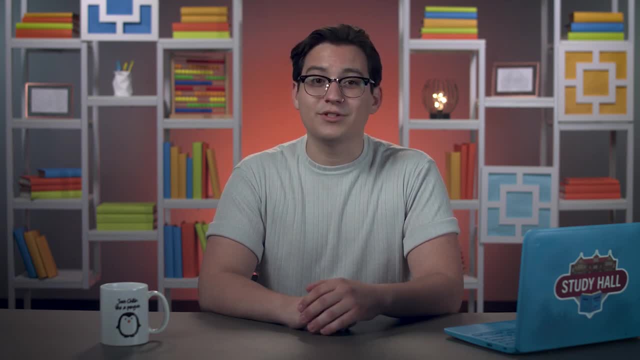 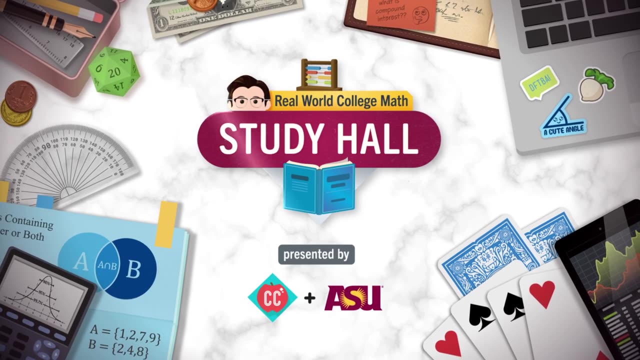 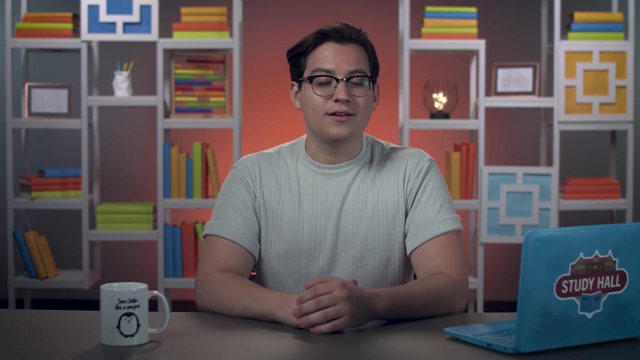 in math and in our world. ask questions and come up with precise answers. I'm Jason Guglielmo and this is Study Hall Real-World College Math. Over the course of our first unit on Set Theory and Counting a lot of the abstract. 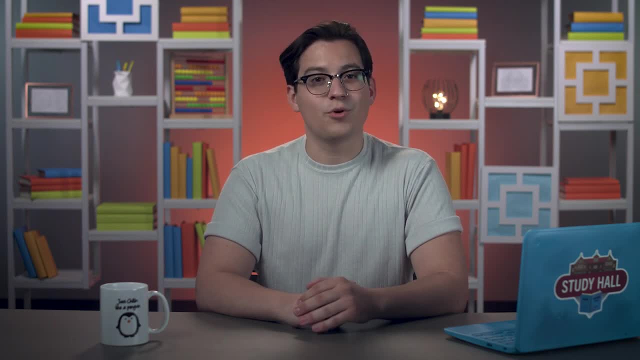 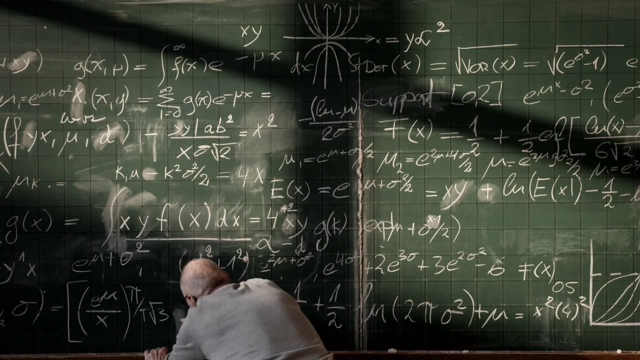 thinking we'll do will give us the tools we need to come up with solutions to more concrete problems, And this might be new for a lot of us. In school, you might have been taught math as sequences of operations or a bunch of calculations you make to get a. 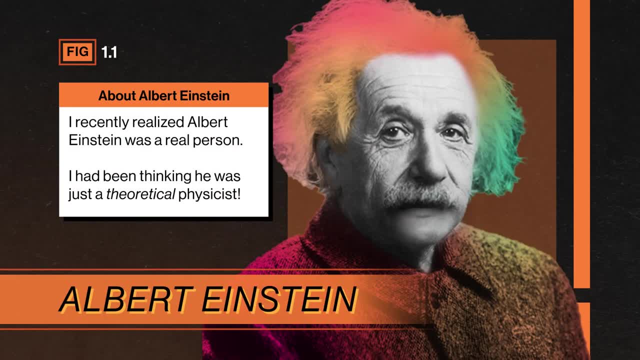 certain answer And sure calculations are important, but, like Einstein said, math is also about ideas, And that's what we're going to talk about today. So let's get to the ideas that we can use to express things in a clear and logical way and combine to 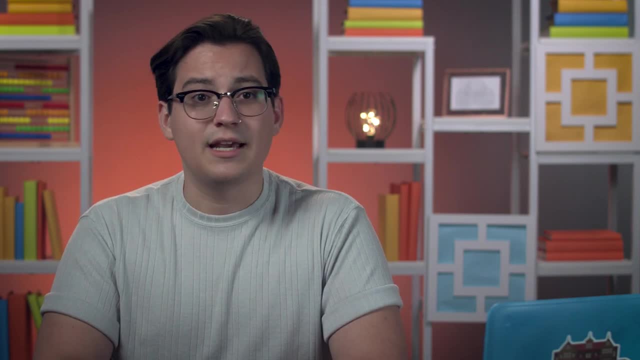 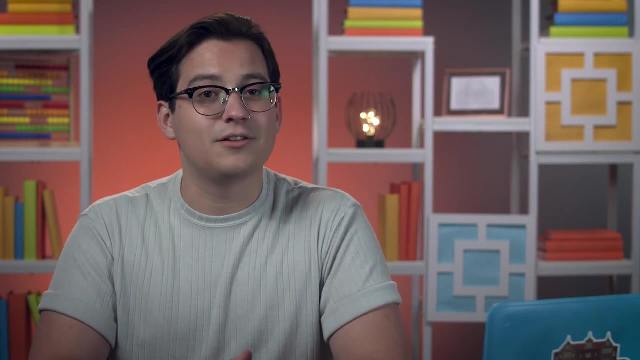 come up with new ideas. So, instead of studying methods or techniques for solving certain problems, over the next few episodes we're going to focus on building a kind of language for expressing mathematical ideas and keeping things clear and unambiguous. And since many mathematical ideas are just 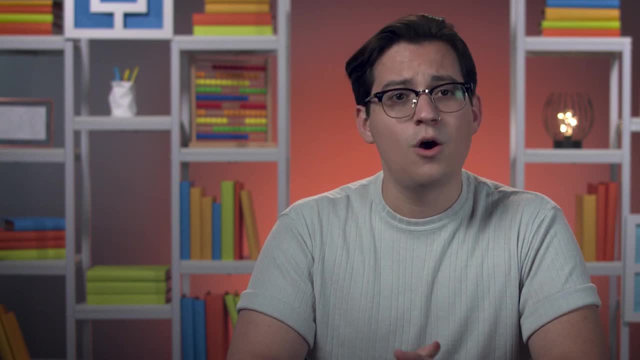 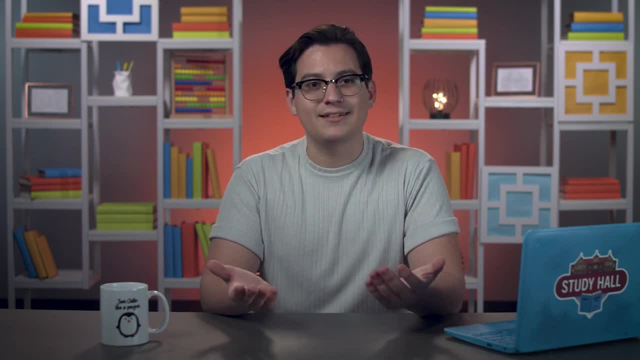 basic set theory we've ever learned. Take the most basic set theory we've ever learned. Take the most basic and important object in set theory. You guessed it: a set. Much like the word in the English Language, a set is a collection of objects. But when we talk about sets in 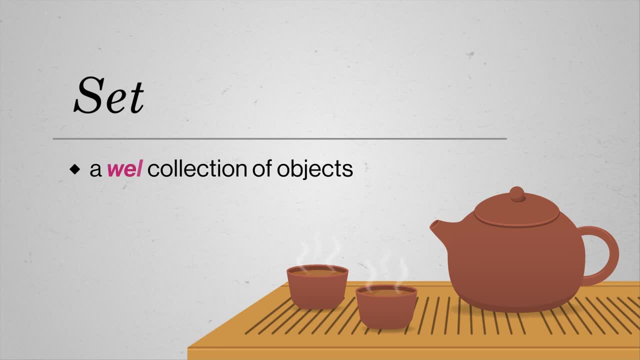 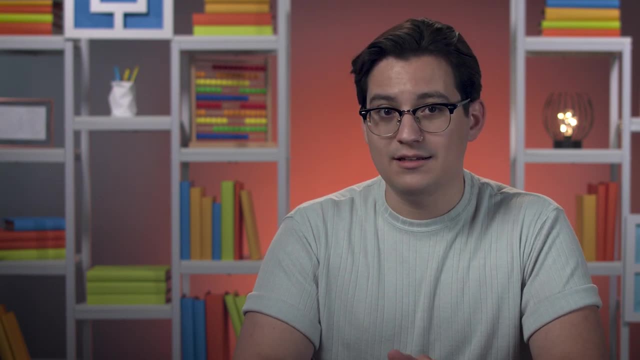 math, we also mean something a bit more specific. We say a set is a well defined collection of objects. that means we can definitively decide whether something is or isn't in a set. And if we don't have a way of deciding, then we don't have a set. 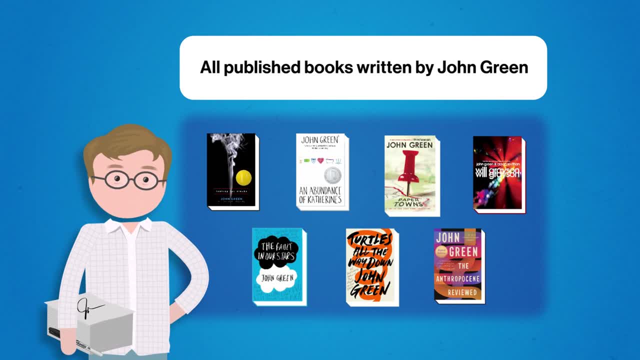 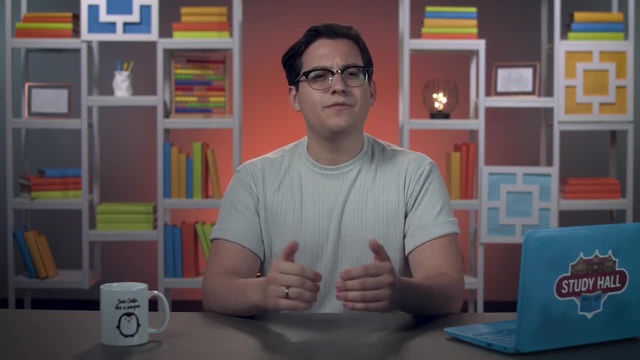 For instance, we could talk about the collection of all published books written by John Green. Either John wrote the book or he didn't, So that's a set. But let's think about another group of things, like the collection of all the best-tasting. 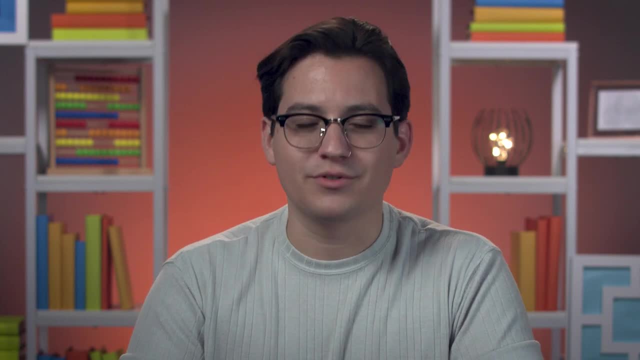 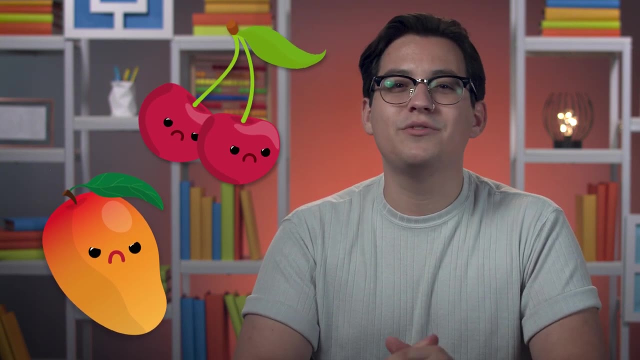 fruits. I'm ready to fight anyone who doesn't think mangoes are some of the best things they'll ever eat. But you might hate mangoes and think I'm ridiculous for not loving cherries. It's hard to argue. there's an objective way to decide which fruits belong in the collection. 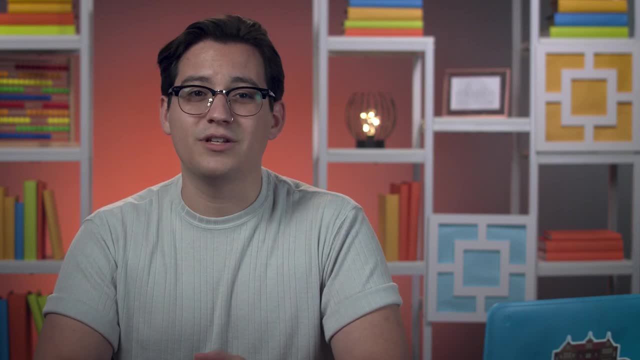 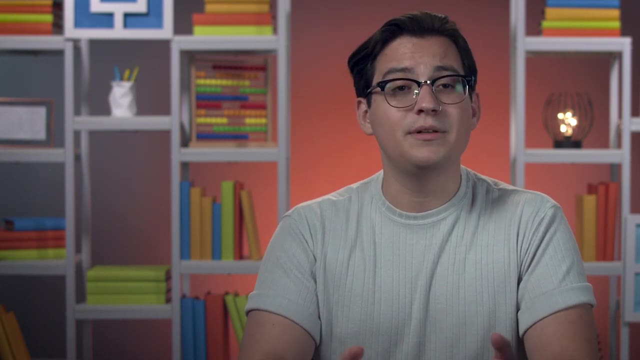 So best-tasting fruits do not make up a set using our precise math definition because it's not well-defined. Now, as mathematicians who need precise and clear language for building new ideas, unsurprisingly, we also have a word for whatever we're putting in the set. 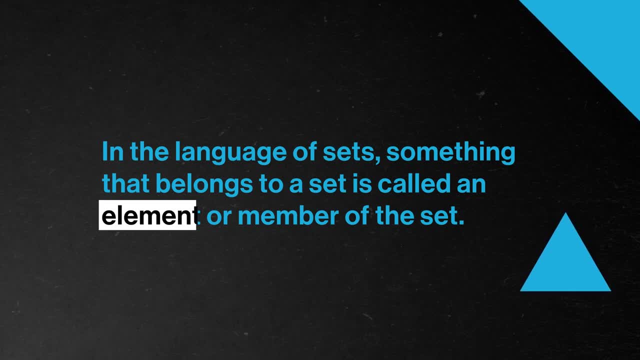 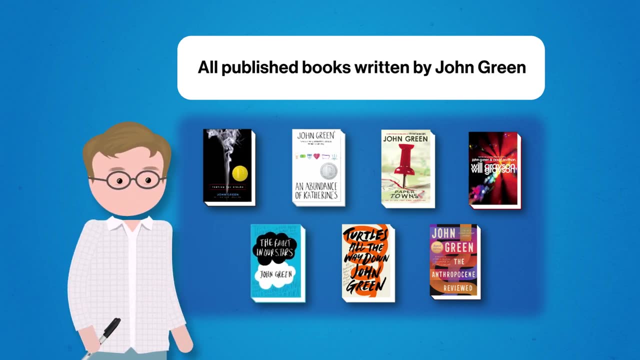 In the language of sets, something that belongs to a set is called an element or member of the set. For instance, the fault in our stars is an element of the set of John Green books, But- an absolutely remarkable thing- is not an element of that set, because John didn't. 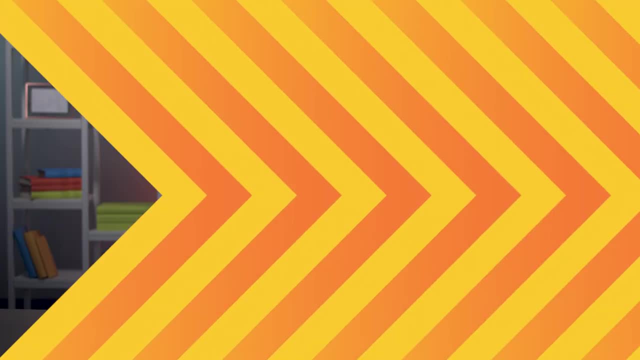 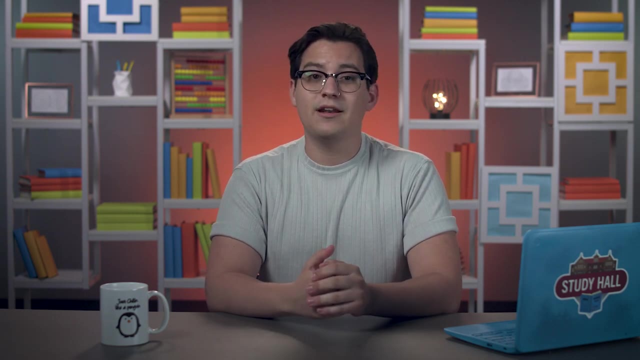 write it, no matter how many people confuse him with his brother Hank. As long as the collection is well-defined, pretty much anything can be an element of a set, But when we're dealing with math, the elements of a set are often mathematical objects like 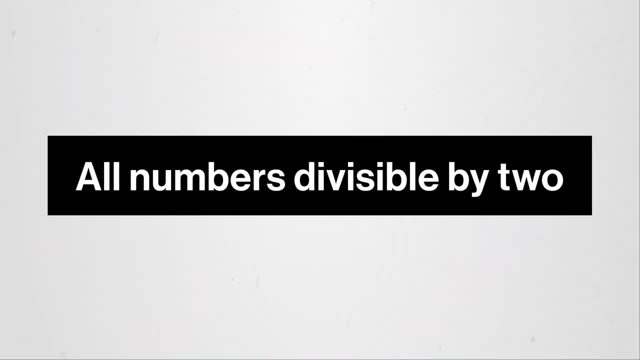 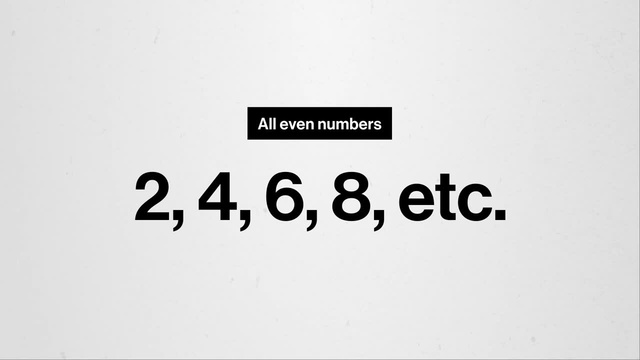 numbers. Let's say, our set contains all numbers divisible by 2, or, as they're more commonly called, even numbers like 2,, 4,, 6,, 8, and so on. Just like our other examples, this set is well-defined, since we can definitively say: 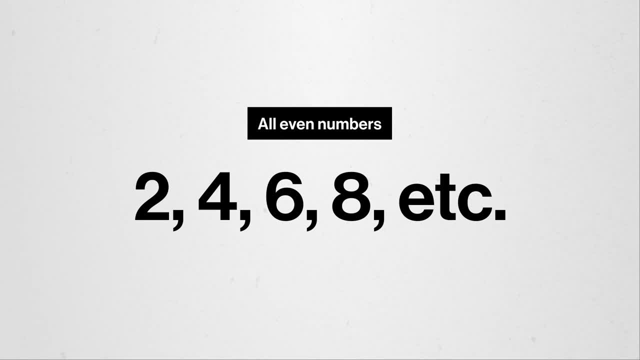 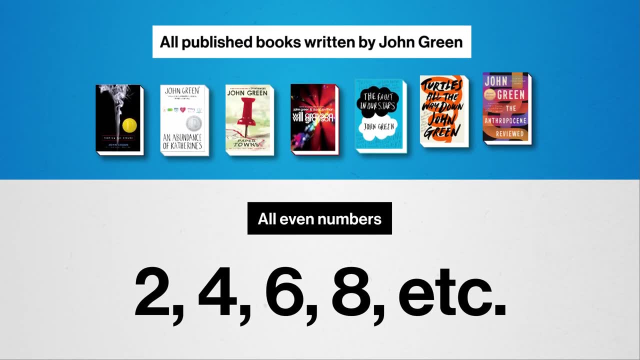 whether a number is or isn't divisible by 2.. But there's something a little different with this set. In our first example about John's books, we know how large the set is because John has written 7 books as of 2022.. 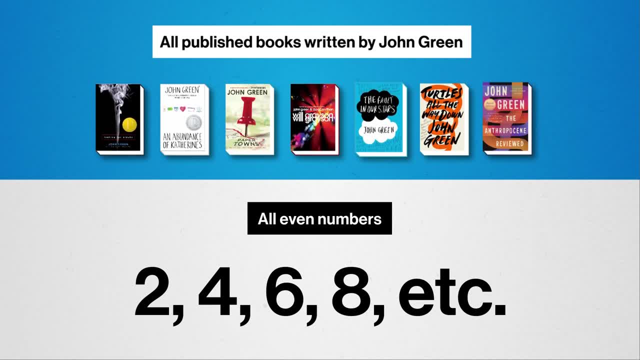 But there are way more than 7 even numbers. We can keep adding 2 to any even number and get more and more even numbers forever. So the set of John Green books is finite, which means we can count the number of elements inside of it and stop counting at some point. 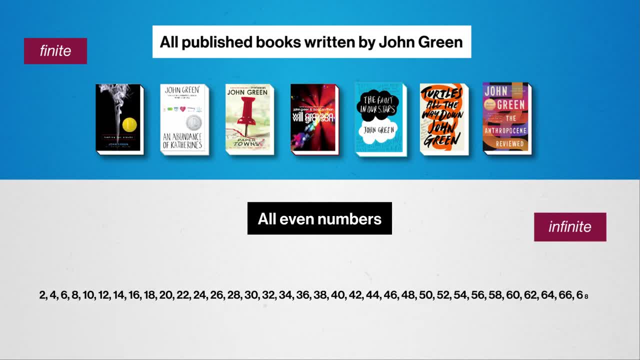 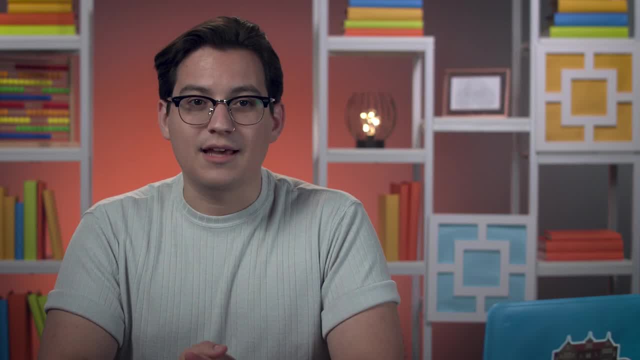 But the set of even numbers is infinite, which means it goes on forever and will never finish counting the number of elements it contains, And that's totally fine. The point here is that there's no limit to how many elements can belong in a set. 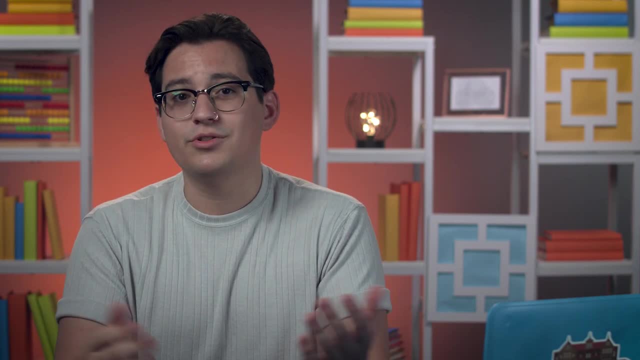 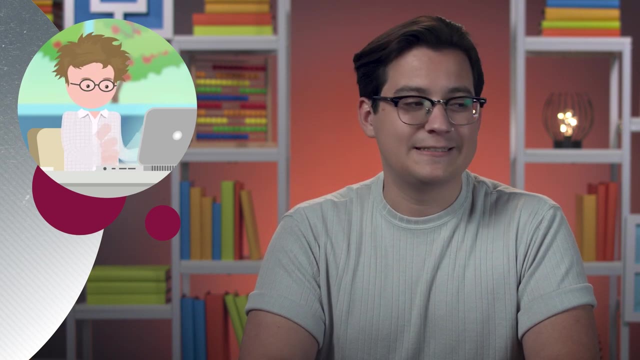 In math, infinitely big sets are pretty common, just like we saw for the set of even numbers. So, John, you've got a lot of work ahead of you if you want to catch up to the set of even numbers. Better- uh, better, get to work. 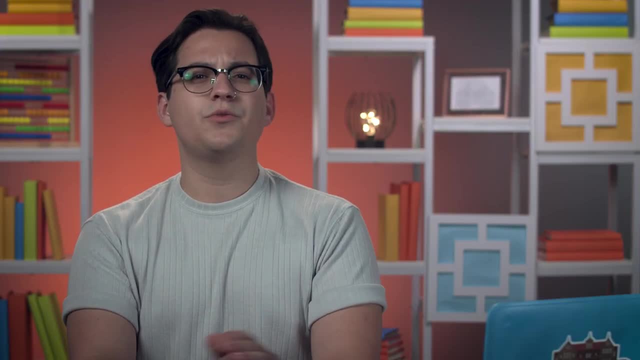 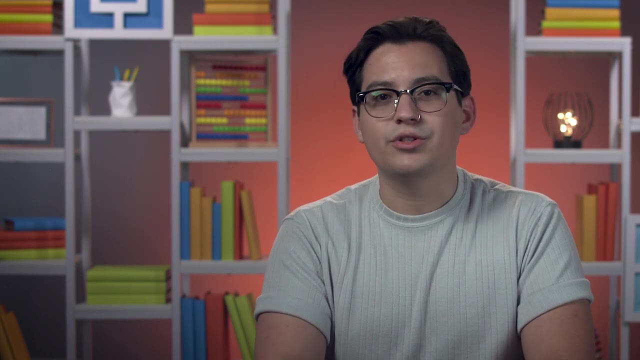 In math we can get really specific about the words we use because we're trying to talk about really precise concepts. Then we take those concepts and fit them together to make something new, just like poets carefully choosing words and ideas to build a poem. 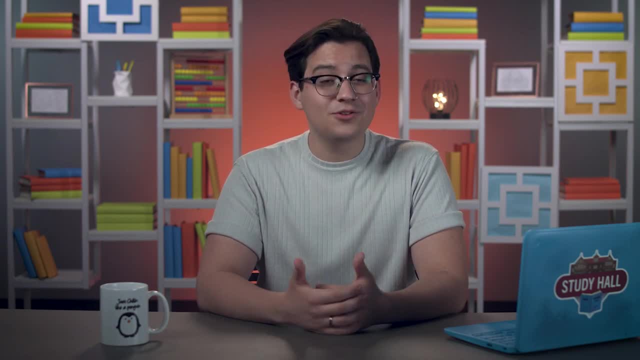 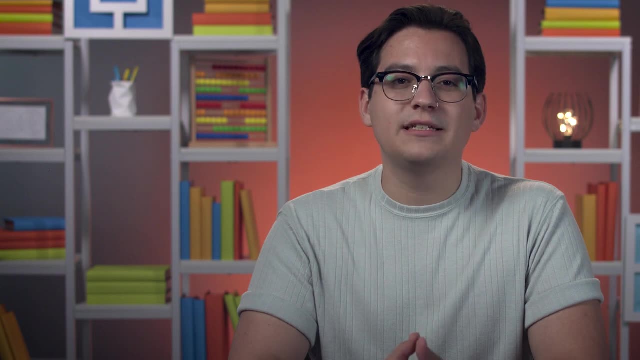 And that's part of what can make math seem like a different language. In fact, it can look that way. So far, we've described sets and their elements using words, but when we're working with sets in math, we'll also need a way of clearly expressing them visually. 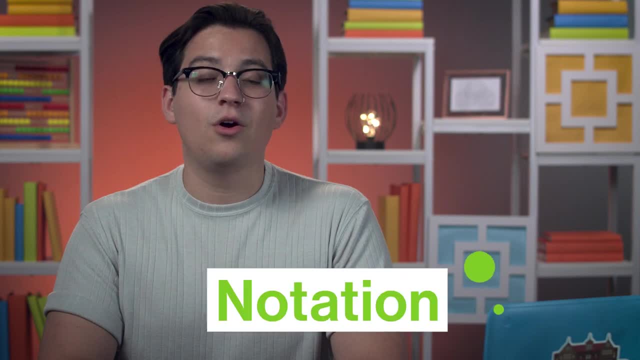 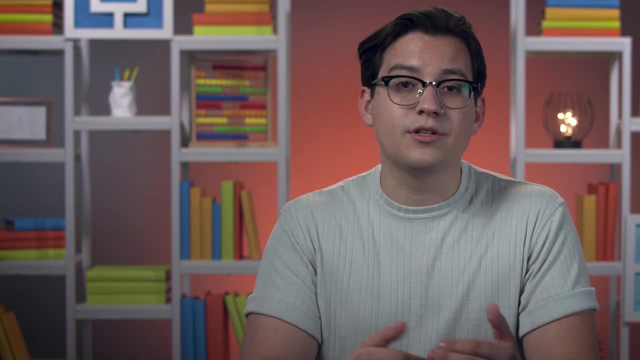 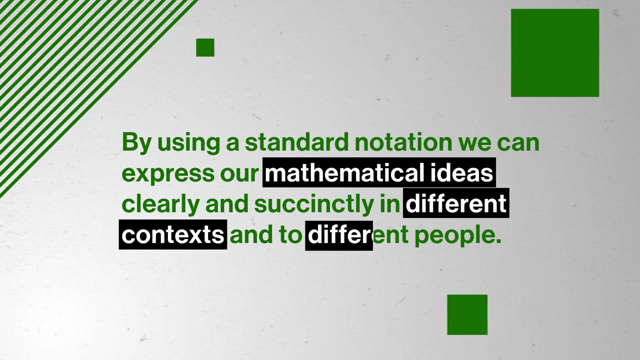 In general, the symbols we use for expressing math concepts in writing are called notation, And the notation might feel a little weird or unusual the first time we see it, But, just like, having specific words helps us communicate. by using a standard notation, we can express our mathematical ideas clearly and succinctly in different contexts and to 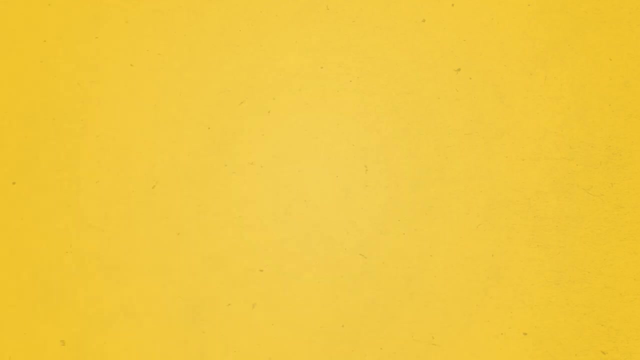 different people. Let's start with a set. The notation for a set is often a set of numbers, So let's start with a set. Let's start with a set of curly brackets. You can think of these brackets as saying: I am a set and any elements I have are inside. 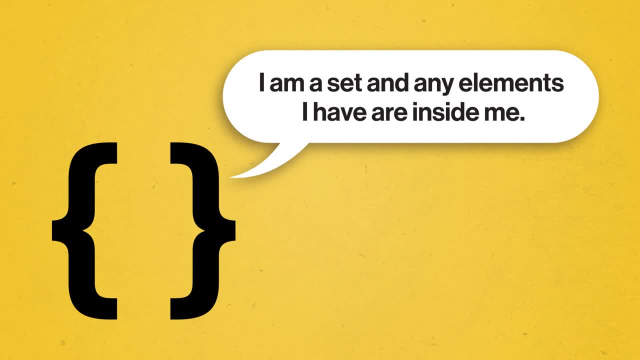 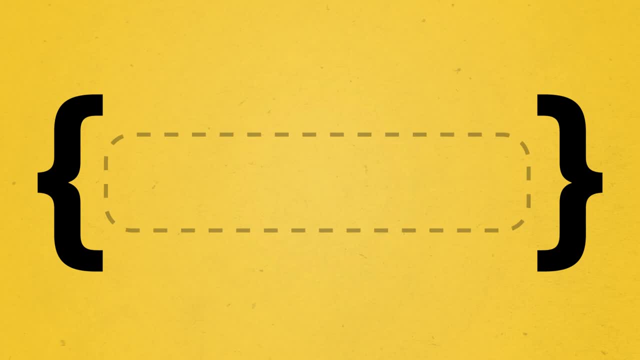 of me, which makes sense, because brackets usually contain something. As for what rule we use to build our set or make it well-defined, one way we describe a set is to use a sentence, kind of like we've been doing. So we could just write whole numbers bigger than 13 between our curly brackets if we wanted. 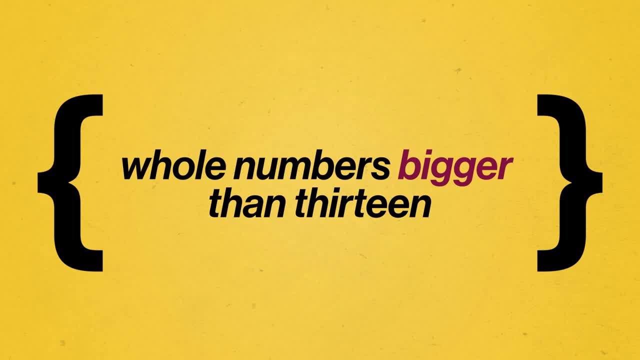 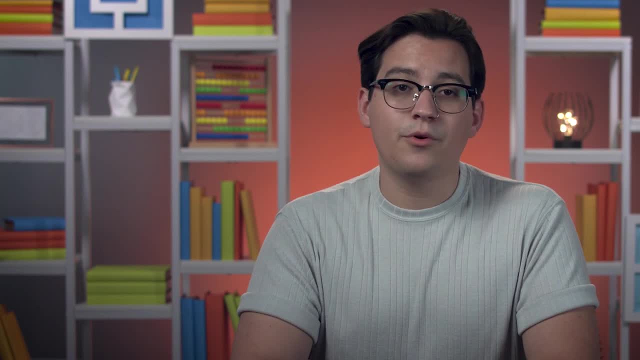 to only talk about numbers bigger than 13 that don't have extra fractional bits, But other times it might be clearer, quicker or even easier, Or even easier to write a set in a different way. if we're going to keep referring to 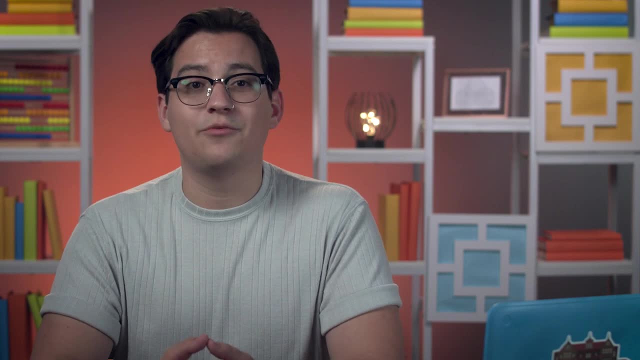 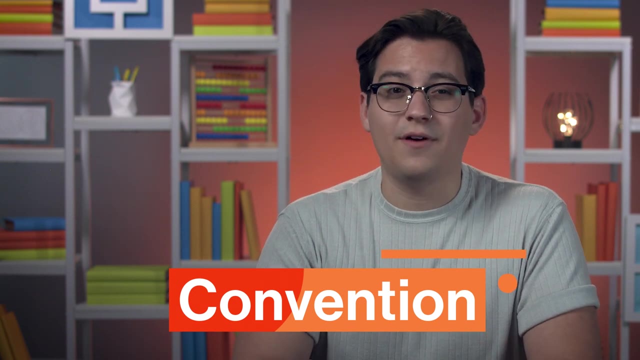 it Like we can assign our set a letter that represents it, so that, instead of writing out the full set every time, we can just refer to the letter. The convention, which is math, speak for rules that people tend to follow, so we all understand. 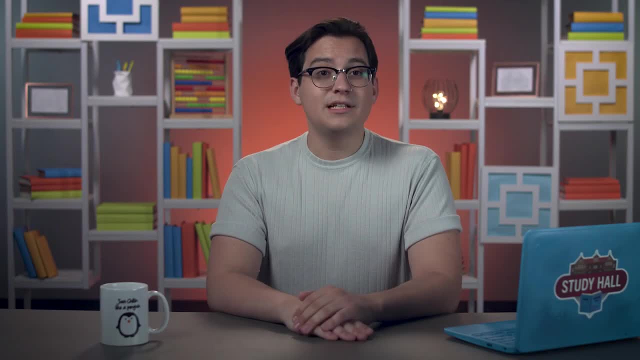 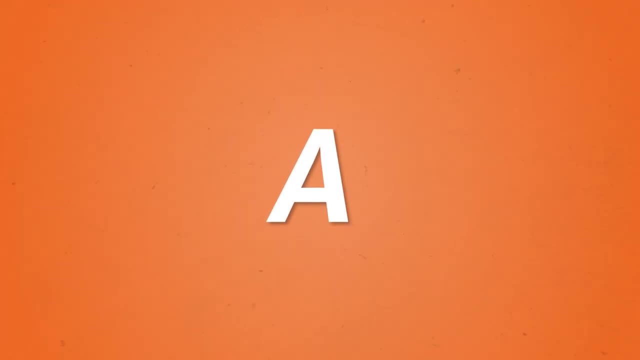 each other is to use a capital letter for describing sets, We still have to make sure that people reading our work later understand what the heck we're saying. So for our set. if we wanted to use a capital A to refer to it at some point we'd have 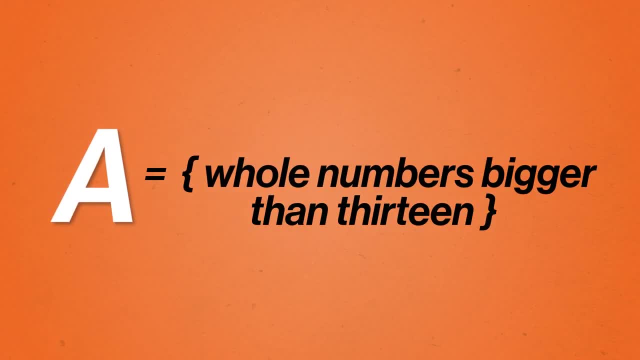 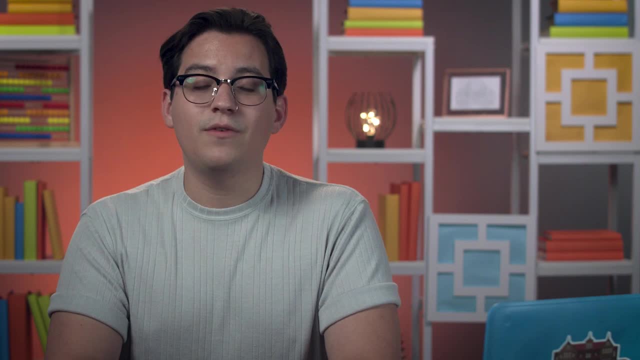 to say that A is equal to our set. After that, we can use A to refer to our set as long as it doesn't have any other meaning in what we're doing. And now that we have a notation for sets, we can move on to their elements. 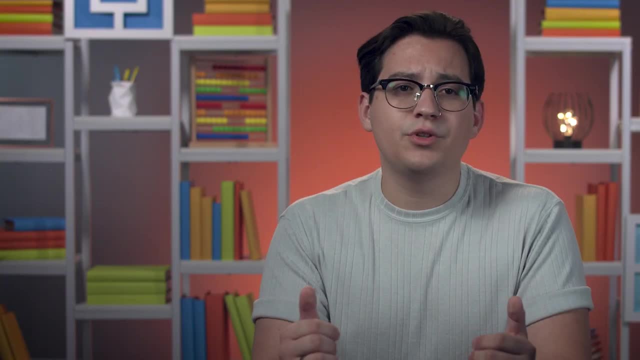 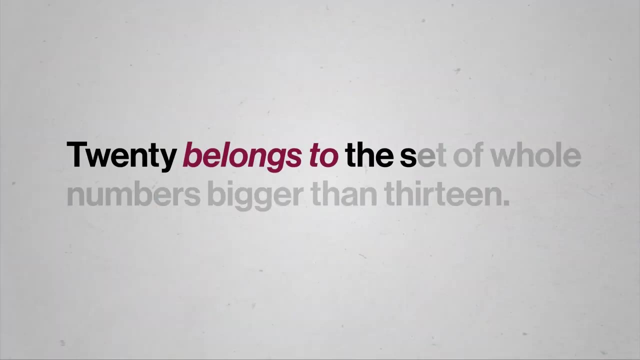 We often refer to elements as belonging to a set And we also have a special notation which means belongs to, which looks a bit like a curvy capital E, So we'd write 20 belongs to the set of whole numbers bigger than 13.. 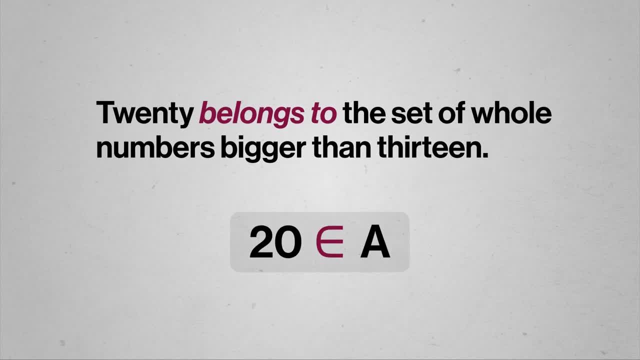 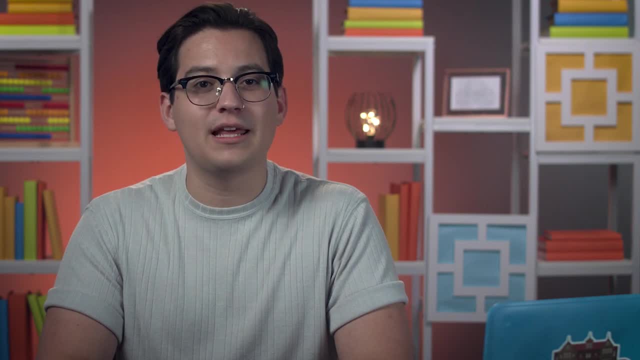 Or we could say: 20 belongs to A, which we know from before, is our set of whole numbers bigger than 13.. In some cases it can also be convenient to write or even define a set by writing out its members inside the curly brackets. 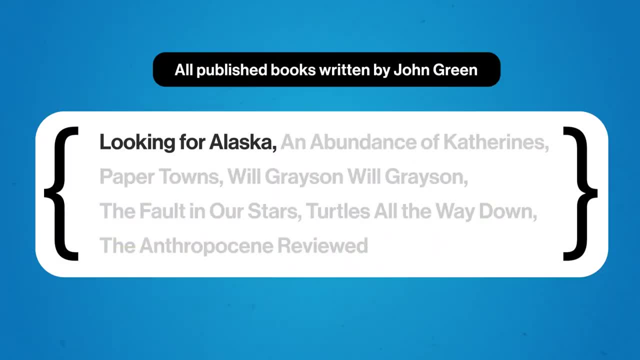 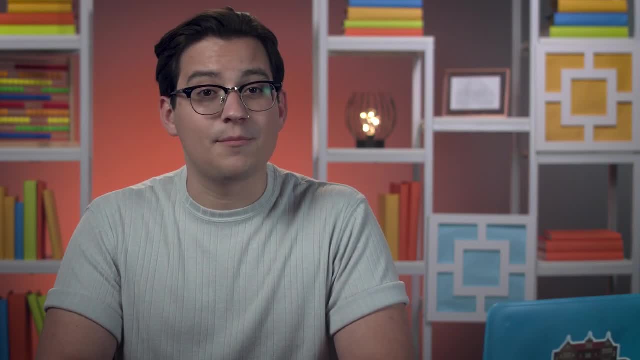 Let's go back to the set of John Green books. For that set we could put the title of each book he's written, separated by a comma, inside the curly brackets, Since this gives us a peek at the members of our set like a mathematical lineup. we 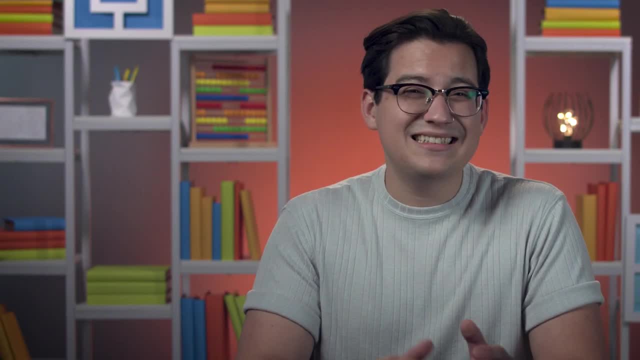 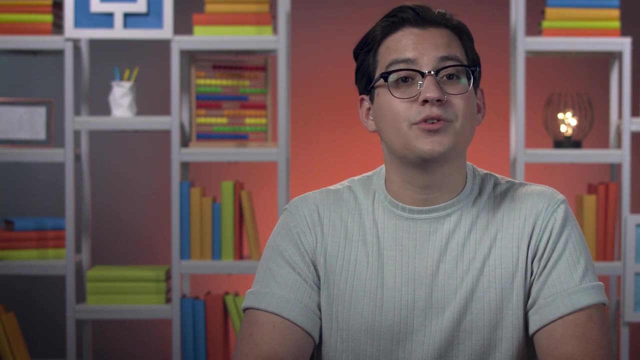 call this kind of notation roster form. But roster form can get a little messy if we have a finite set with a lot of elements or an infinite set, like for our set of even numbers or our set with numbers greater than 13.. 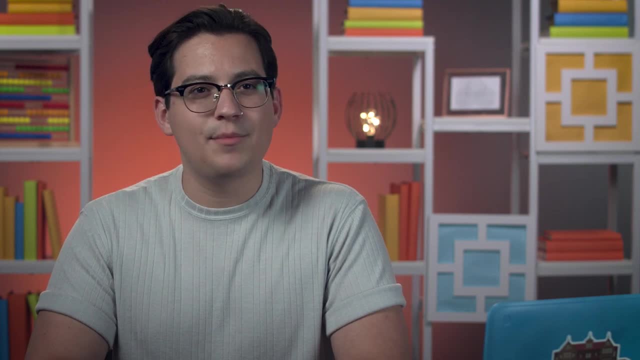 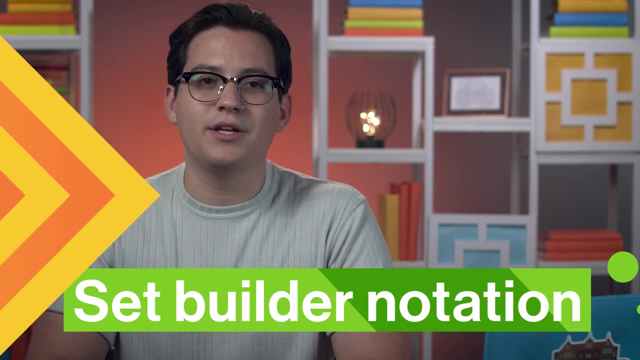 So, especially in situations where our set is hard to describe in a short sentence, we can use a mathematical statement to define or build a set. This is called set builder notation. To use set builder notation, we start off inside the curly brackets and take some symbol. 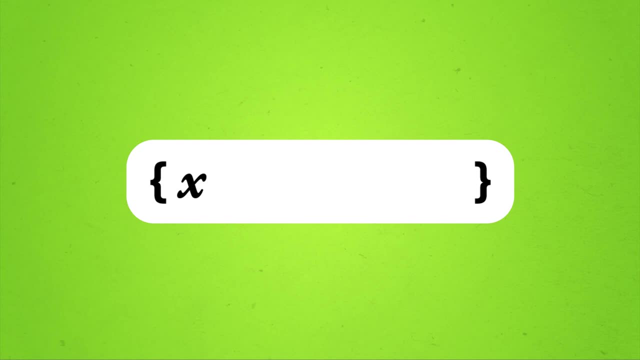 like the lowercase letter x to stand in for any arbitrary element of our set. Then we draw a vertical line and write out the conditions that the elements satisfy, Or in other words, what has to be true for x to be in our set. 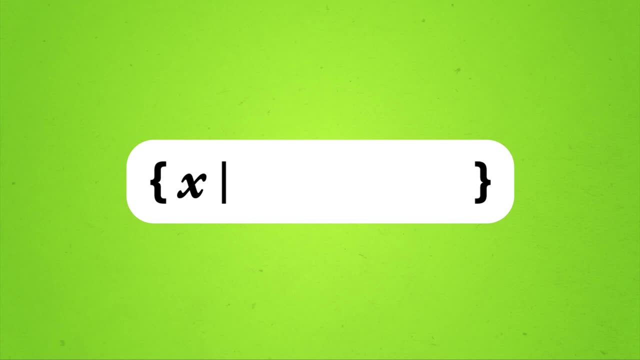 If we're trying to describe this set in a simple way, we're going to need a set of numbers bigger than 13.. To describe the set of all whole numbers greater than 13,, we say two things. One, that x is a whole number, which is the same as saying x belongs to the set of whole. 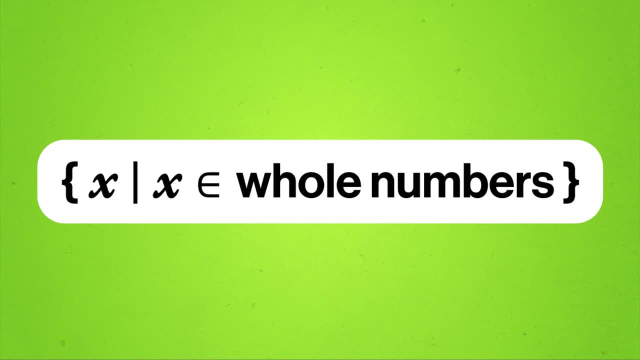 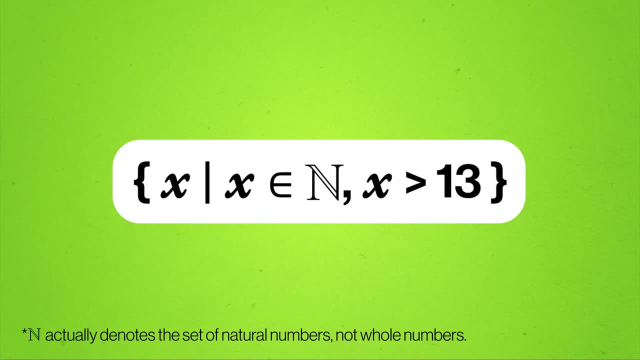 numbers That set actually has its own special math notation in the form of a fancy letter n. Secondly, we write that x has to be greater than 13. This is a different condition from our first condition, so we separate them with a comma. 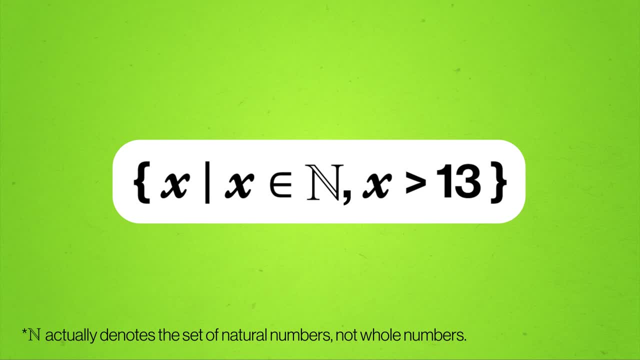 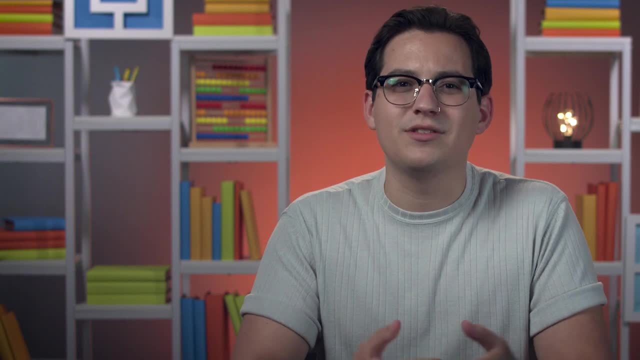 just like we did for set elements. This way, someone could read this notation and build the set based on the conditions we listed. Now, that's a lot of ways to describe sets, And you might have some questions like: why use the letter x for the elements of our set? 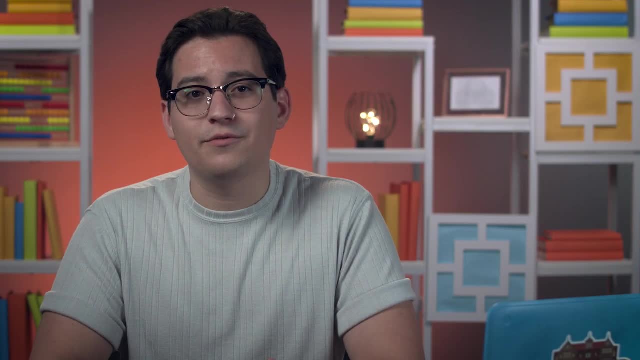 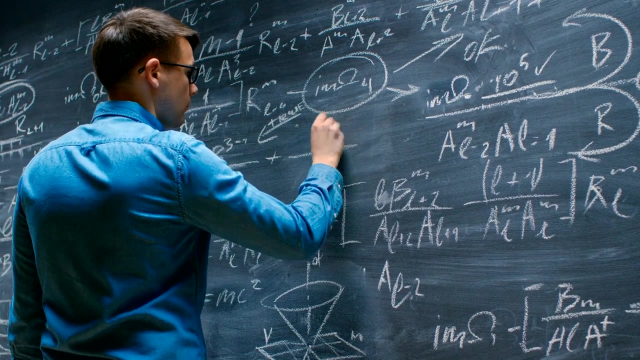 And what's with the big fancy n? These kinds of questions often come up on first contact with any type of math notation. Just like a language, what can feel strange and unintuitive becomes familiar the more you use it, even if the original notation or language seems made up. 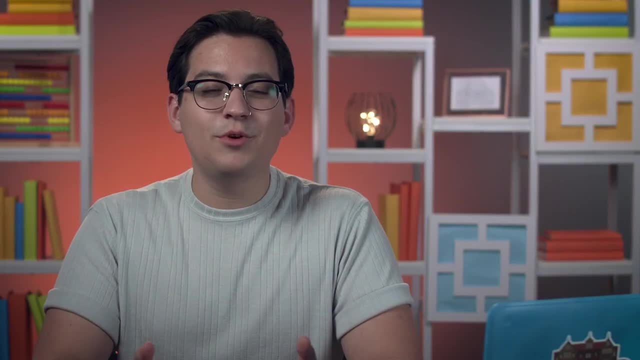 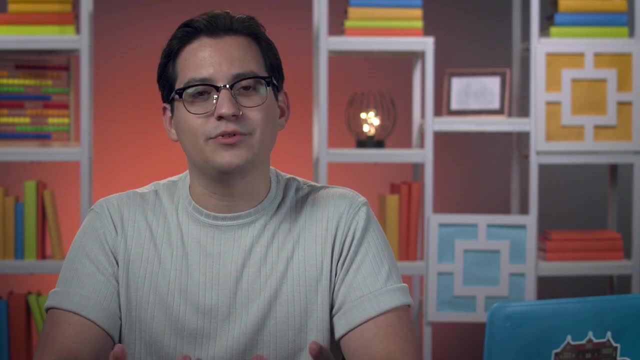 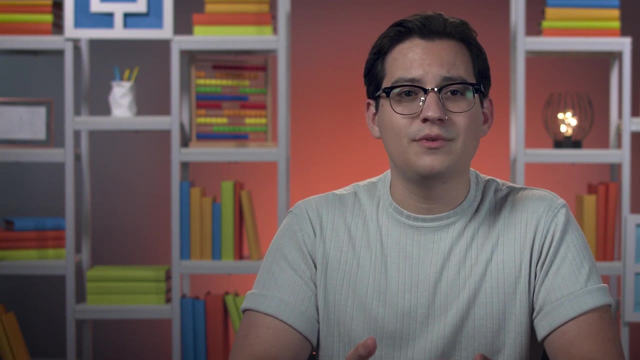